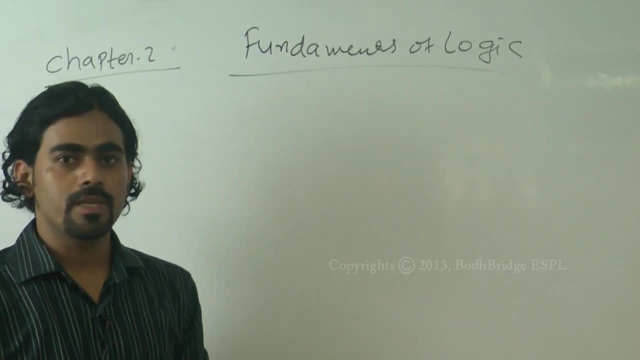 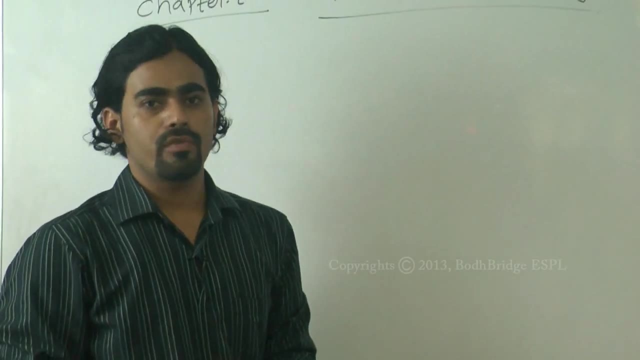 the premises. what are the premises, how we can use different kind of premises, what will be the disjunction, conjunction, what will be the usage, tautology, contradictions, and then, at the end, we are going to learn about the quantifiers, of course. So now in. 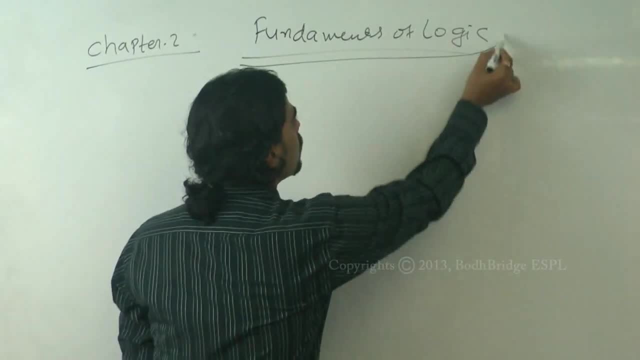 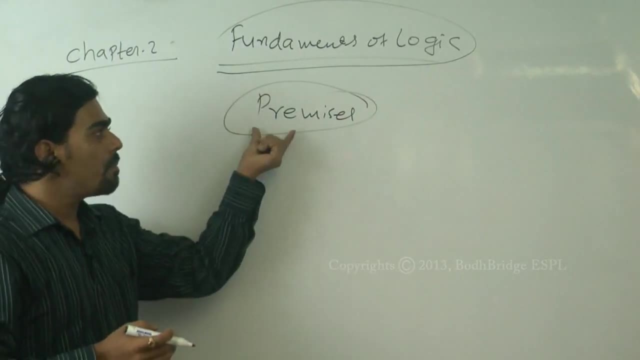 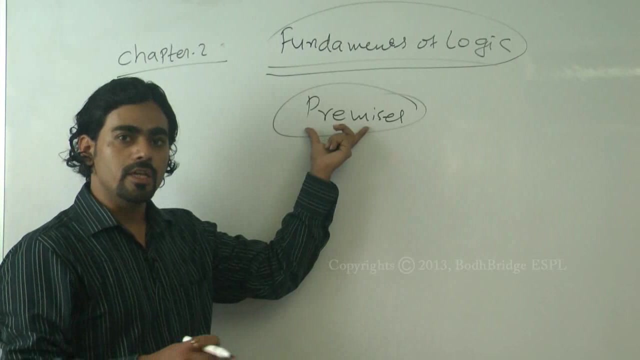 this logic also depends upon the sets. A starting of the logic always starts with the premises- Premises. So this premises is nothing but the basic statements, which can be either true or it can be either false. It cannot be both, So this premises can be either. 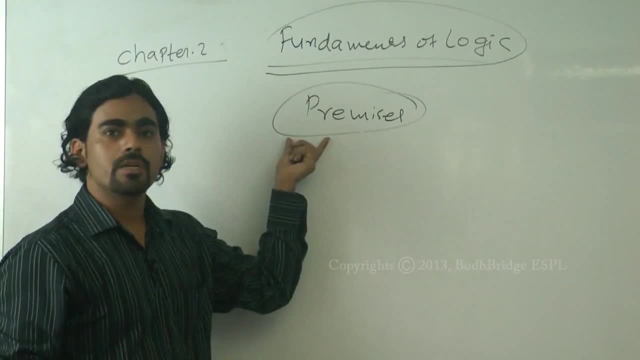 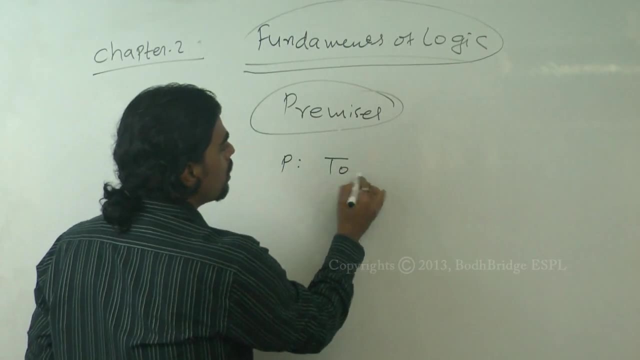 true or can be false. It cannot be. So these are the most basic statements, is there? These are premises. So now for this premises. what is there? Let us suppose we have a premise called P, if today. So there are two premises. I have taken P and Q. Today is Sunday and 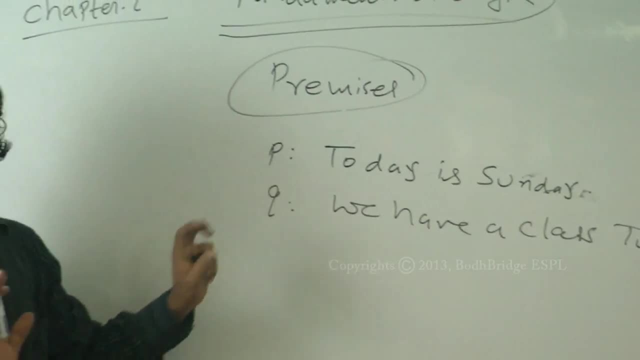 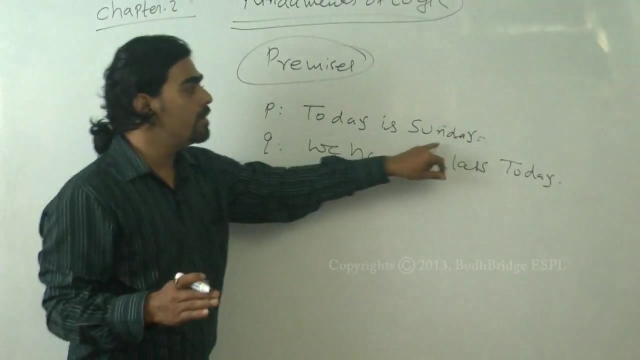 Q: we have a class today, So this we have taken randomly. So I am not telling that whether it is a true or false, but it will be either true or false. Either today will be Sunday or it will not be Sunday. It cannot be both. Today is Sunday as well as not a. 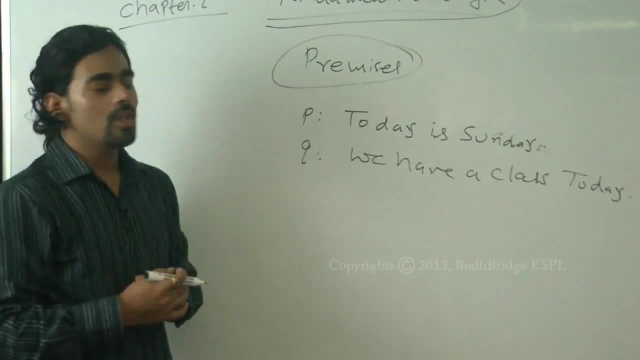 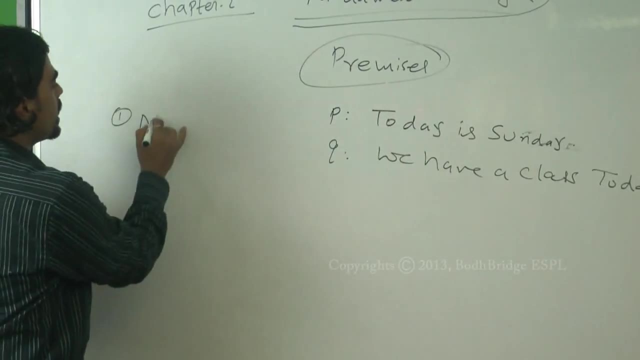 Sunday: It cannot. So that are the basic statements here. premises are there. So either it can be true, it can be false. So in the fundamental of logic, basically we are going to represent first one negation: How to represent the symbols. Firstly, we have to learn it. So how to find? 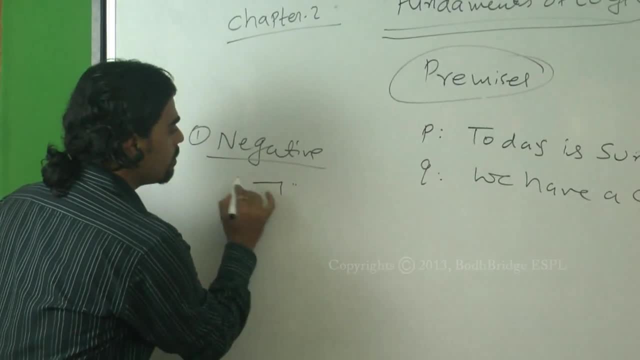 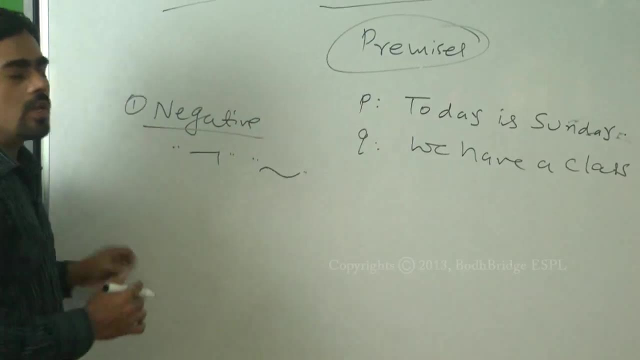 a negation of a statement. So negation is going to be represented with these symbols, or sometimes with this symbol also. they used to write. So negation we are going to do, let us suppose, P negation. So if you are going to write a negation of a statement, 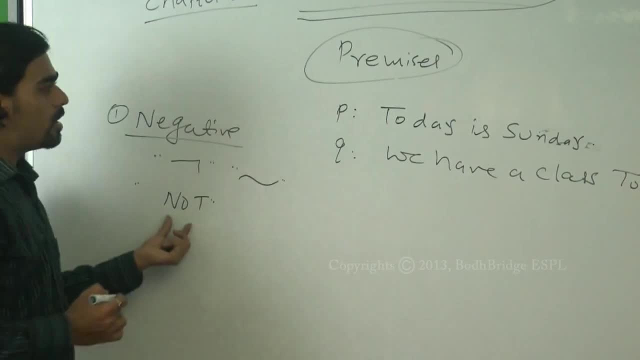 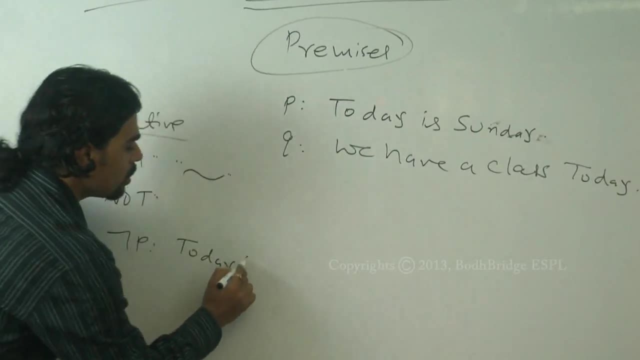 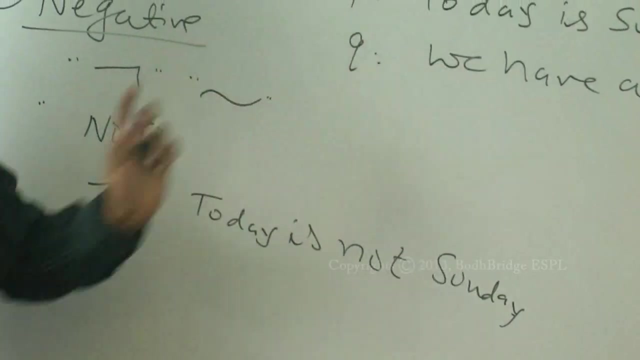 so that put a statement not word, not word in the given statement. So P they have given today is Sunday, So not of P will be today is not a Sunday. So basically we are just going to add this, not word into the given statement at the appropriate place. We are. 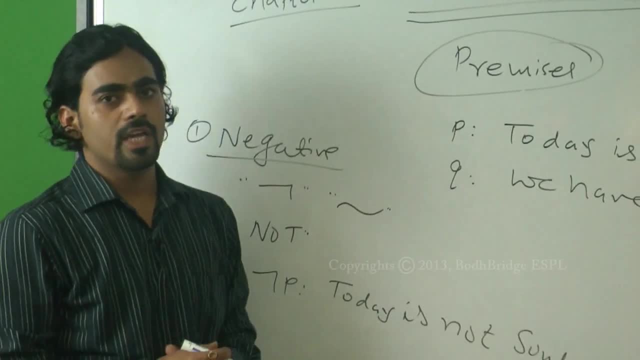 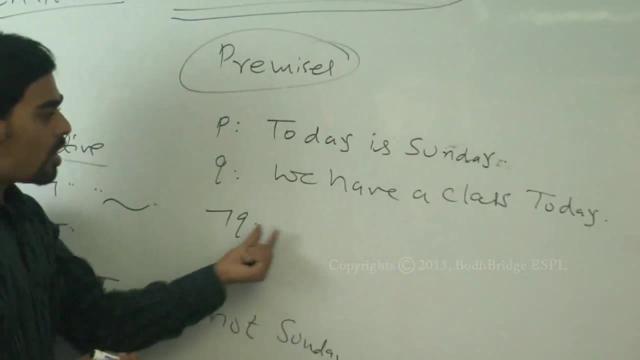 not bothering about whether it is a true or false. Simply we have to write the negation of the statement. Similarly, if I ask, what is the negation of this? Q means we have a class today. So not of Q means we do not have a class today. or we do not have a class today, or we. 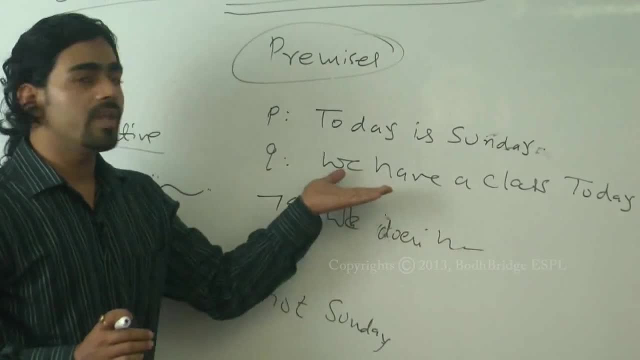 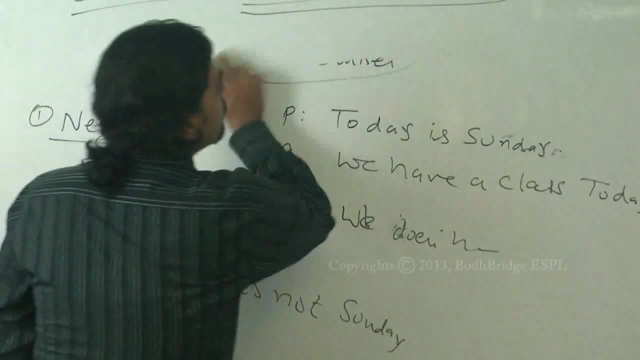 have not a class today that also we can write. We are not bothering about the meaning of this statement only now, not, we have to negate the given statements. So that was the negation. Second is the conjunction If, for, not only if. I am talking about the truth table. So 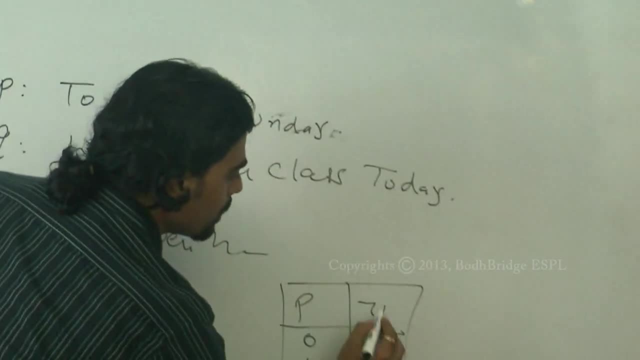 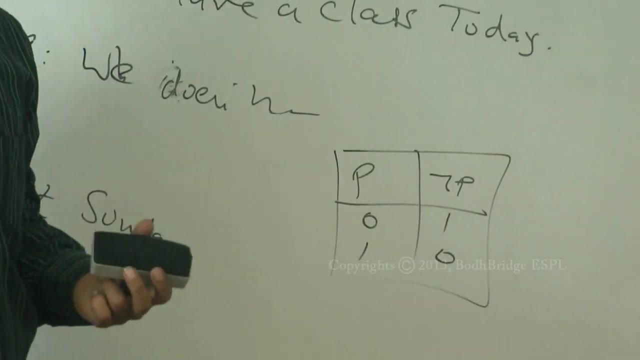 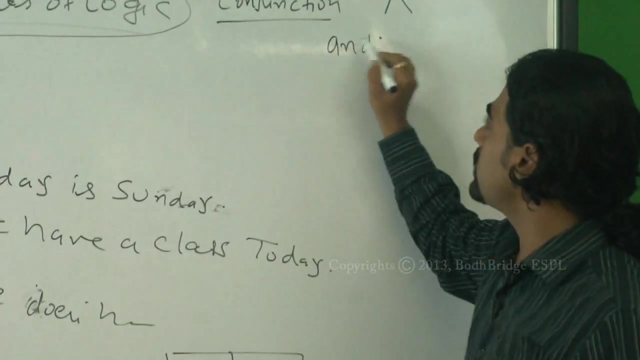 if this is a P, So either it will be true or false. So not of P will become one and zero the truth. table Now conjunction. conjunction means it's the symbol. conjunction means whatever things are common in both. this is going to be used using the AND statement conjunction. 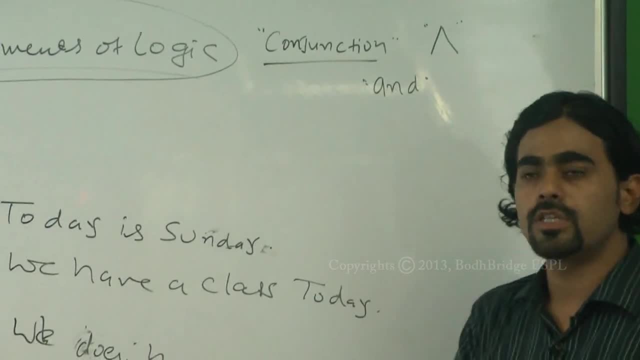 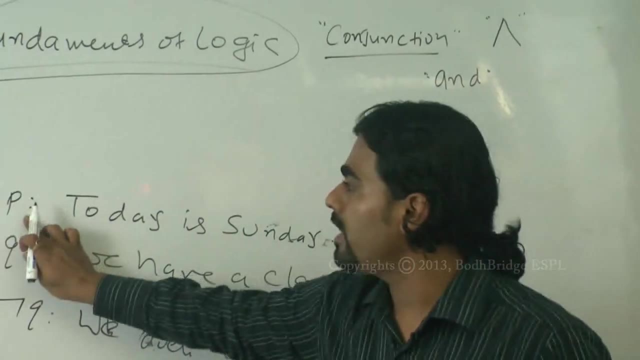 of two statements means joining of two statements. what is the common in two statements? so that if two statements are there, so conjunction is going to be used to add this to a statement using the AND word. so here P is there and Q is there, so conjunction of this is will. 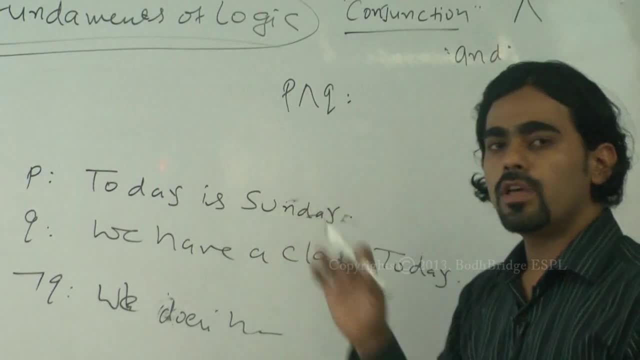 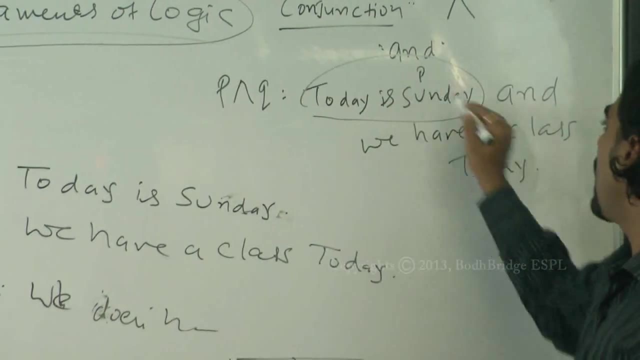 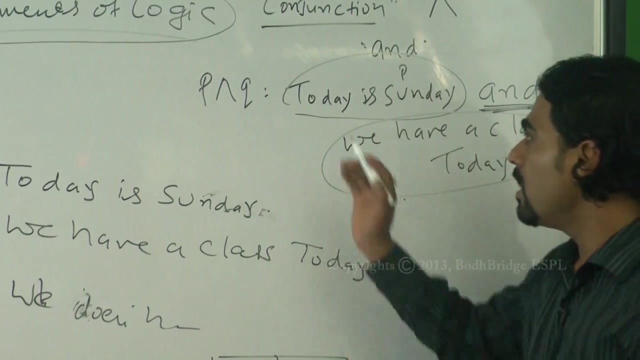 be: write first statement, put a AND word, then put the another second statement. so what will be there? simply, we have copied this paste, copied P, and here we have a copied Q, and in between we have put a word, AND. so that's what you have to do, it, nothing more than that. now, 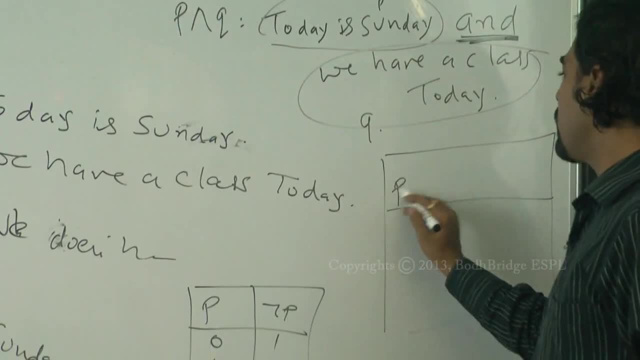 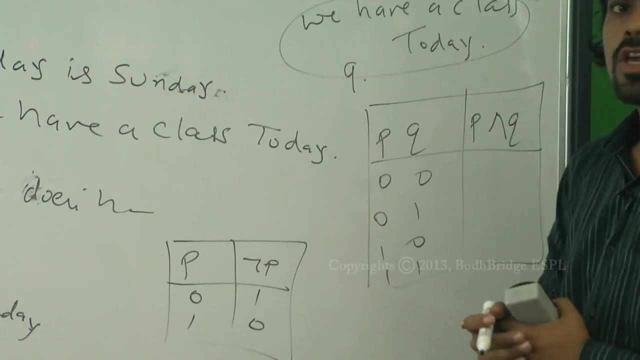 if you are talking about the Venn diagram, what will be the Venn diagram? this is my P and this is Q: 0 0 0, 1, 1 0, 1 1. this junction of this. how to write this junction? so I told. 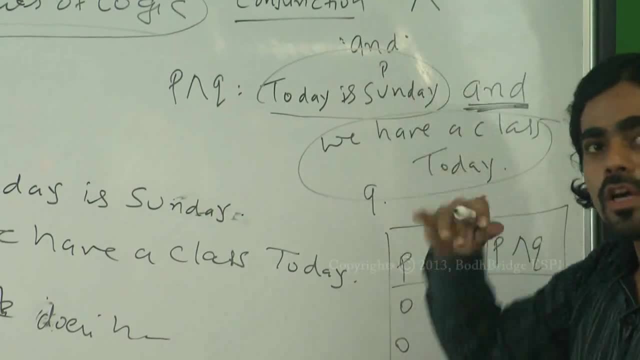 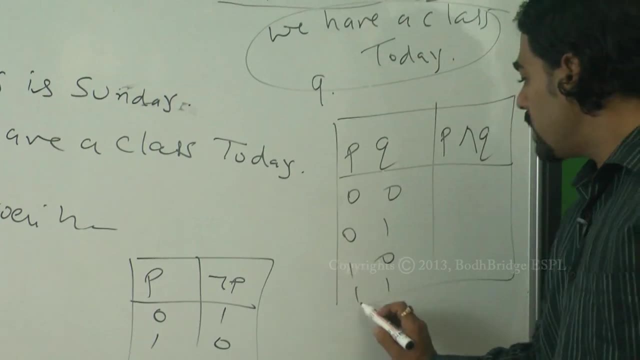 if this is a And word, so AND word always talks about. if both are true, then only it will become true. so disjunction, conjunction, will become only true when both of these are going to be true. so P is true and Q is true, then only it will be true, otherwise, every time it will be false. 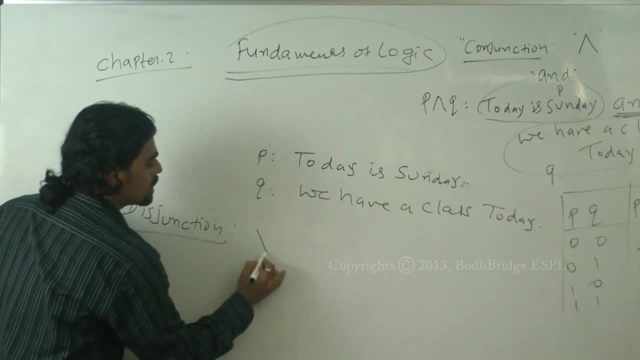 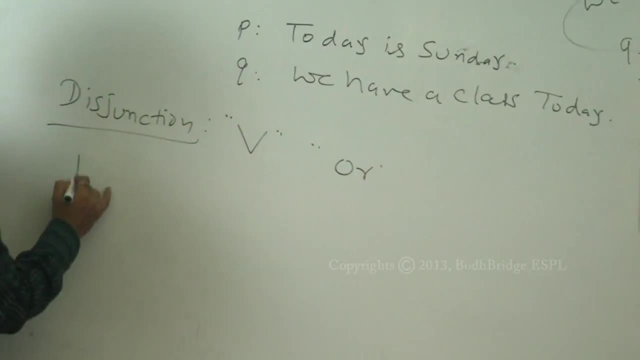 so these things you have to keep remember. disjunction: same thing like this: here we are going to use the word OR. this is OR word, you are going to use it. so means, if you are going to write P. disjunction of Q, we are going to write. 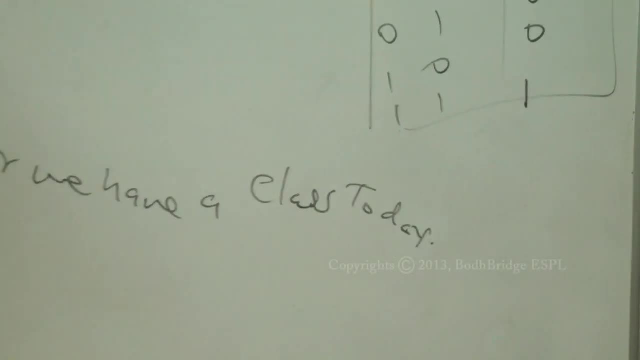 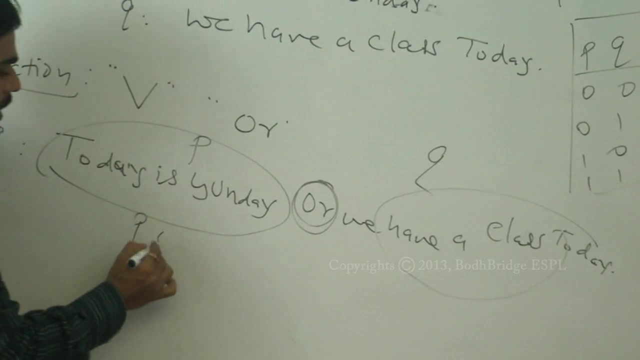 This. So only we have not done anything. this is my p, this is my q, only this or word you have put in between the two statements So we can write p or q. that's it. So this is a disjunction. 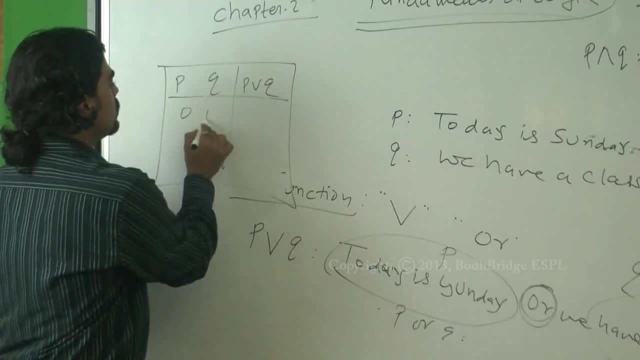 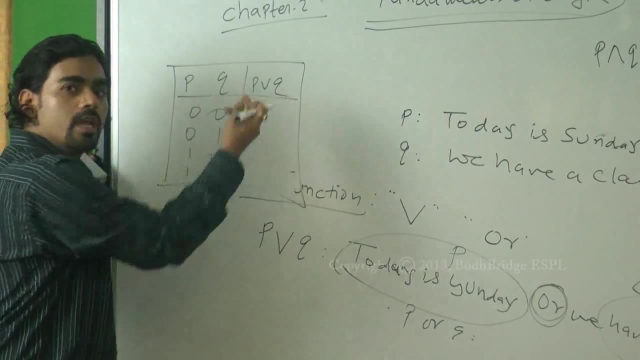 If you are going to talk about the truth, table 0, 0, 0, 1, 1, 0 and 1, 1.. So what will be the conjunction of this? Conjunction of this is nothing, but if any one of this is true, my statement will become: 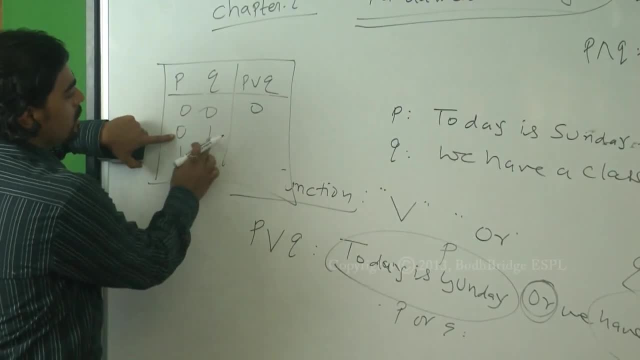 true. So here both are false. so it will be false Here. just see 0 and 1.. 1 is true, it will be 1.. Here also 1. And this: both are true, 1.. So this is my disjunctions. 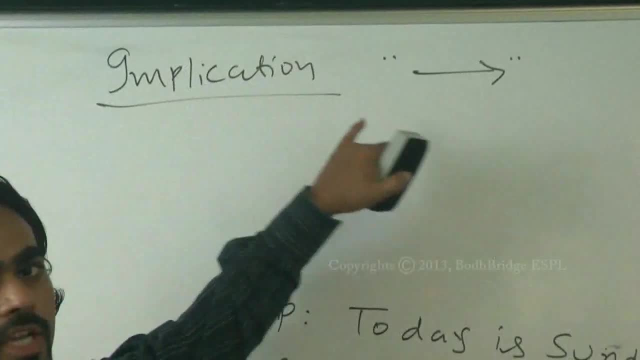 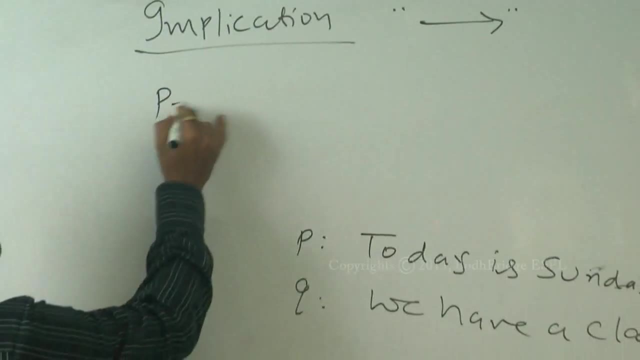 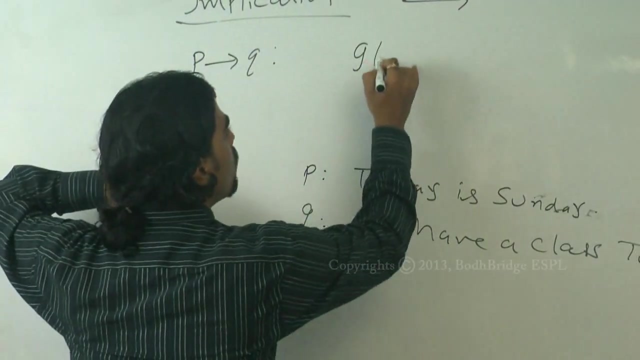 Now. next is the implications. The implication is going to be represented with this symbol. This symbol is going to be used to write the implications. Now for implication. if you have written p to q, so how to write this? To write the implication, we are going to use the word if. then, 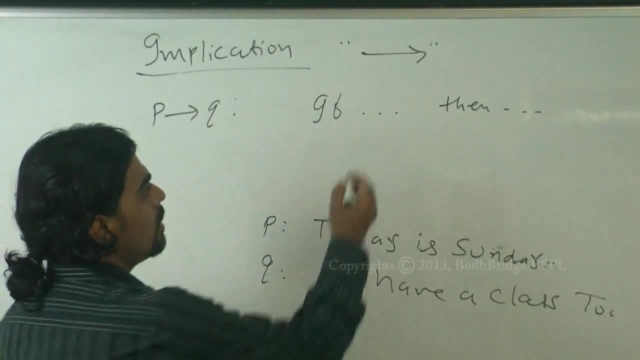 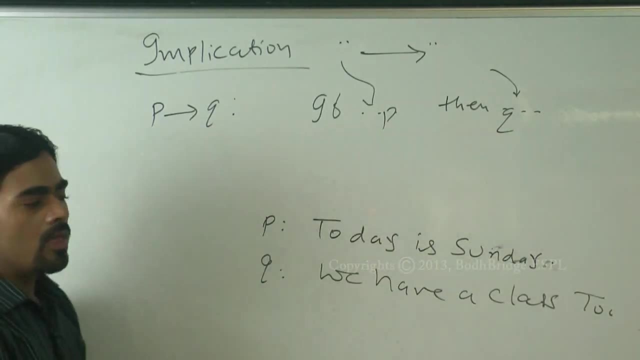 If implication sign is. So basically just write: if, then here left-hand side of this you write, here right-hand side you write, means here p and q, means if p, then q. So for this statement, if I am going to write p to q, so what to write? 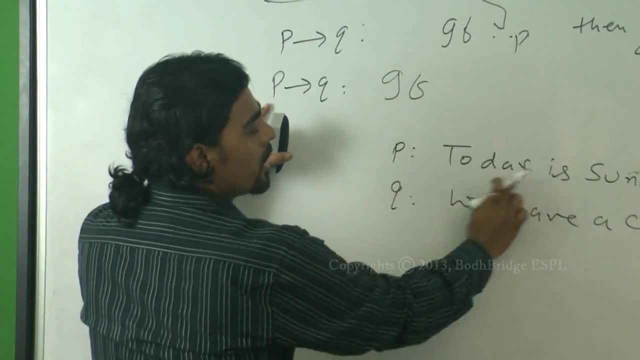 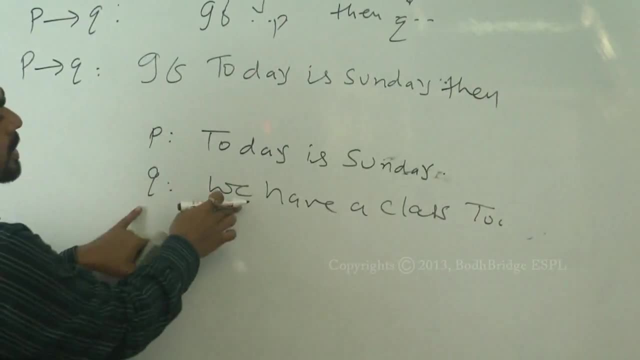 Firstly, you will put a word. if then write p- p means today is Sunday, right Now once again- then you have to write. then then q, q is there. just copy this q and paste it. We have a class today. 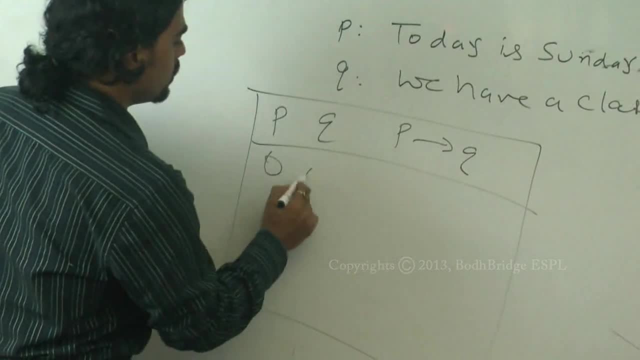 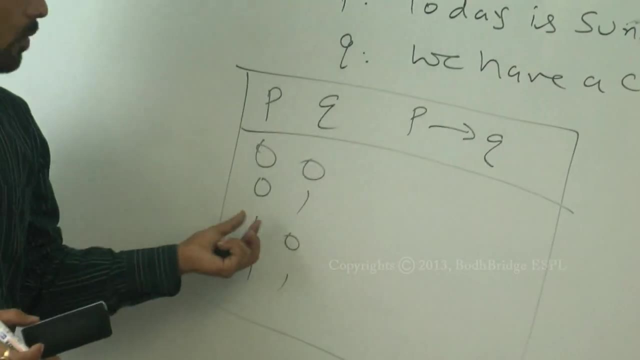 So that is a statement. We are going to write truth table for this. so 0, 0, 0, 1, 1, 0, 1.. How to write the truth table. So this statement will be true only when first statement is a true and second one is a false. 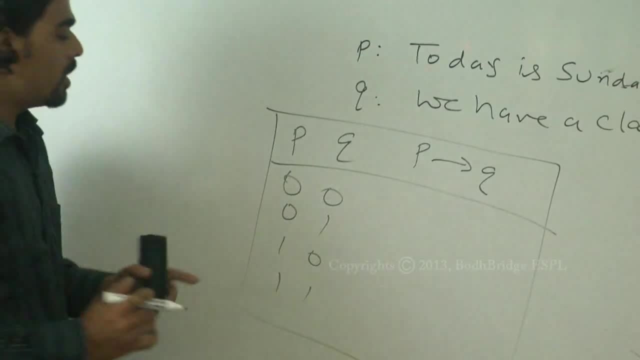 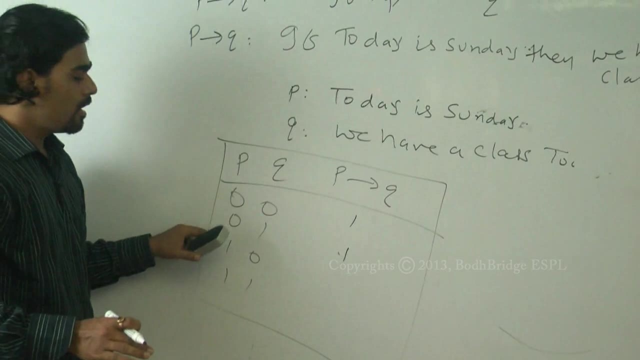 then this given statement will be false. otherwise, it will be true every time. It means 1, 0 to 0,. it is a true. this is also a true. this implication is going to be false only when p is a true and q is false. 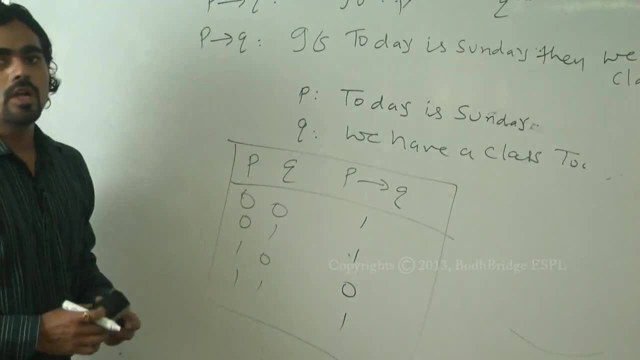 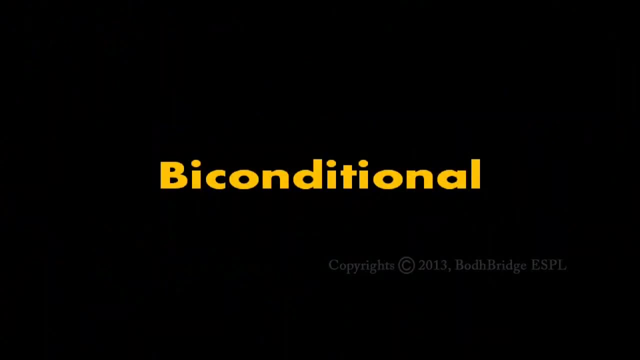 So this is the only condition when this will become false. otherwise, every time it will be true. So this is how we are going to do this Now. next one is the biconditionals. So biconditionals is going to be represented with this symbol, both way. 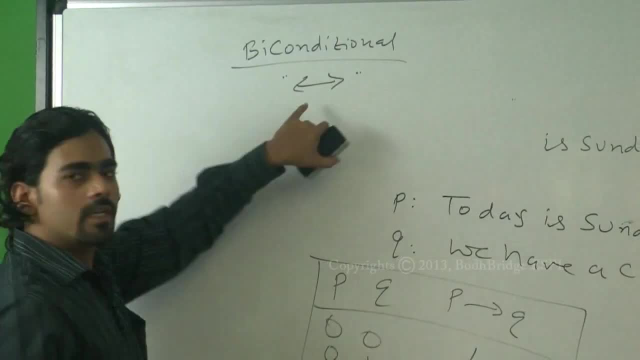 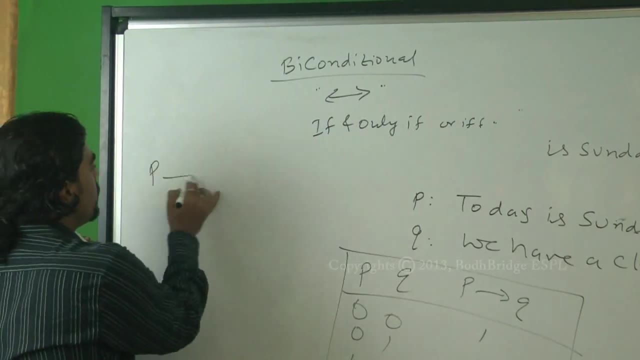 So this symbol is going to be write: what is the keyword value for this? If, and only if, both the things you can use for the biconditions. So if you are going to write p, implication of q, so it will become today is Sunday. if 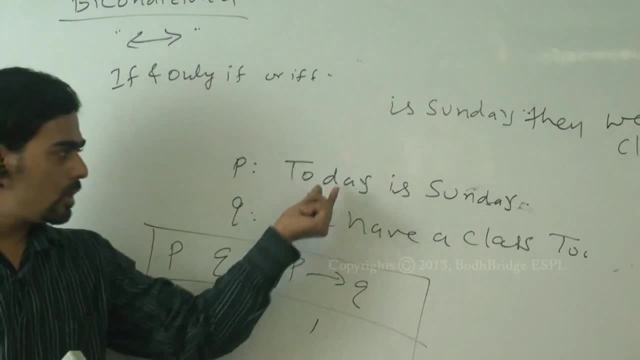 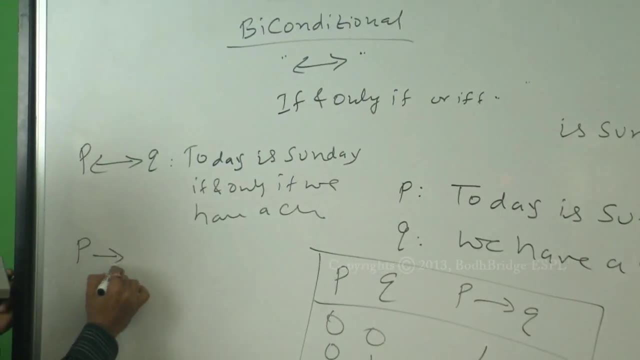 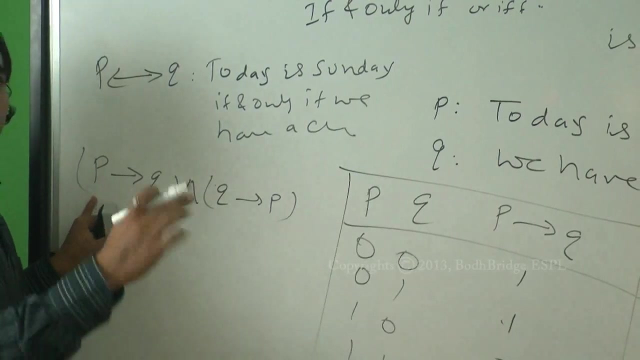 and only if we have a class today. Okay, Today is Sunday, if, and only if we have a class today. So now we can write. So this biconditional is nothing, but we can write p to q. conjunction of this. This biconditional is nothing but this: a to b and b to a. 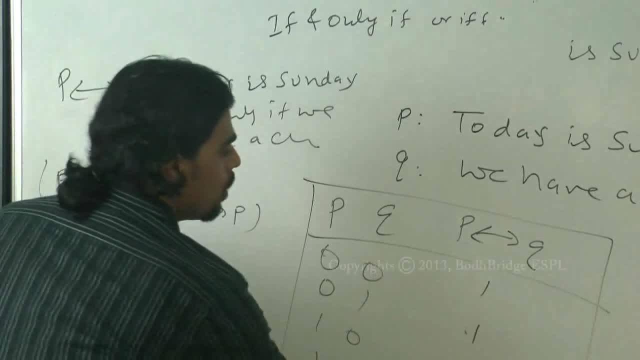 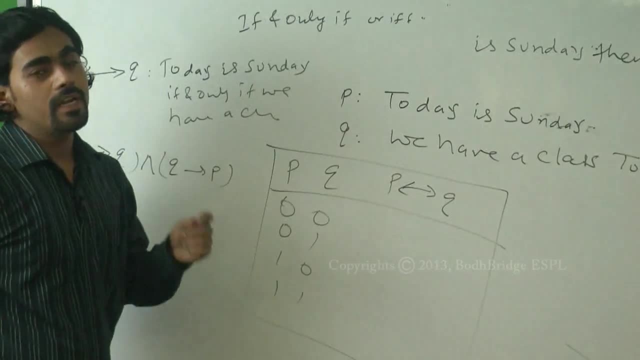 So that is a biconditionals. If you are going to write a truth table for this, what will be the value here Truth table. if you are going to write So here, it will be true only when- if both are there in the same state. 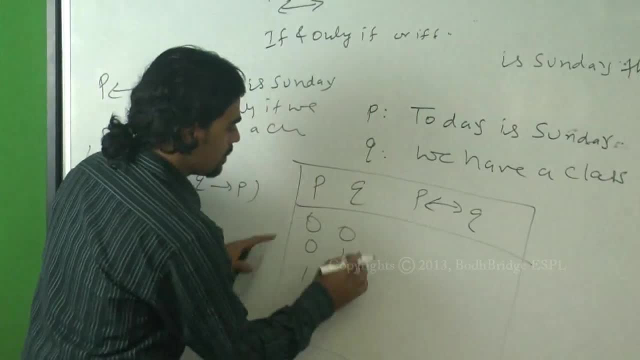 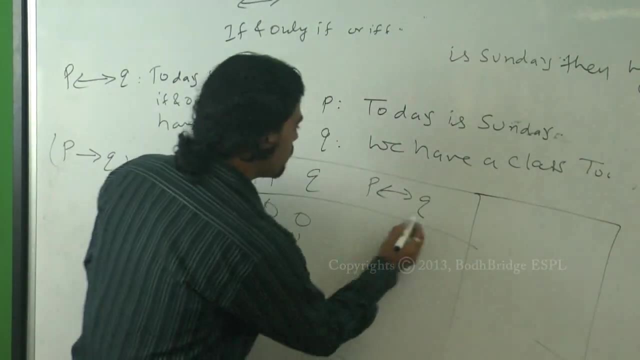 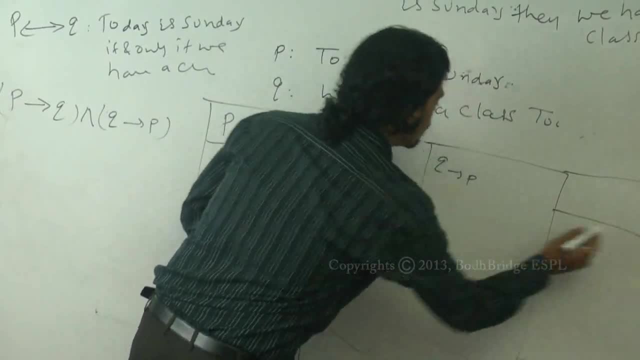 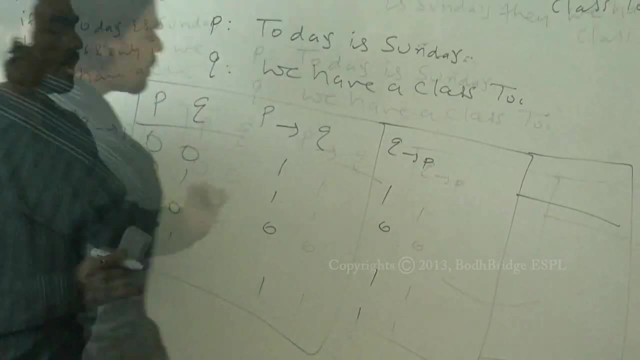 p to q. firstly you write it, Then you write q to p And take a disjunction of this, both. So what will be? p to q? So this will be 1, 1, 0, 1 and this will become 1, 0, 1, 1. intersection of this intersection. 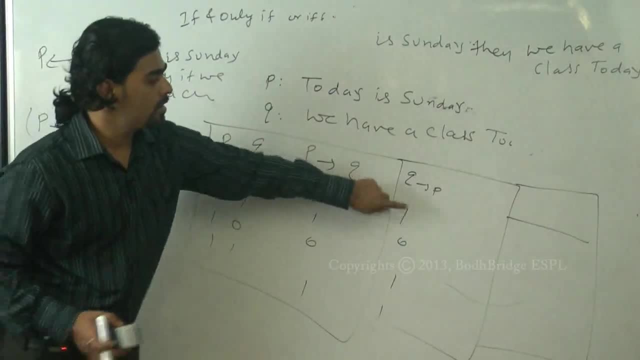 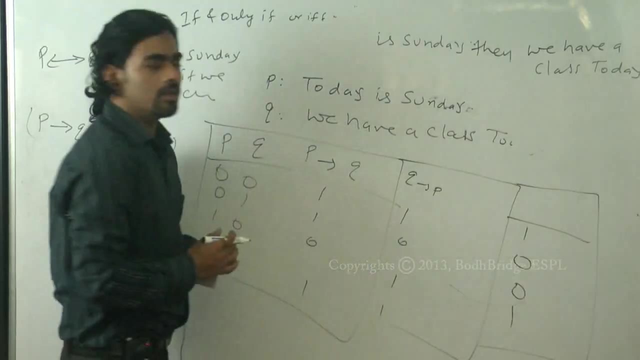 of this, or conjunction of this: 1, 1.. So this will be 1. 1 0 0, 1. 1 0, 0.. 0, 1, 0 and this is also 1,. so that's what I told. it's nothing but my biconditionals. 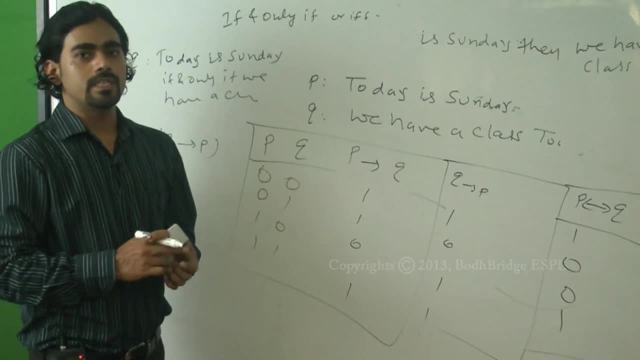 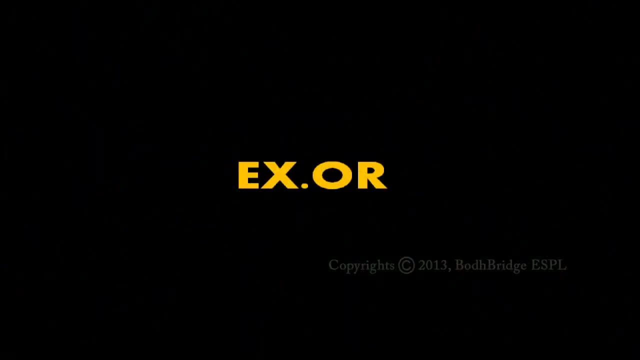 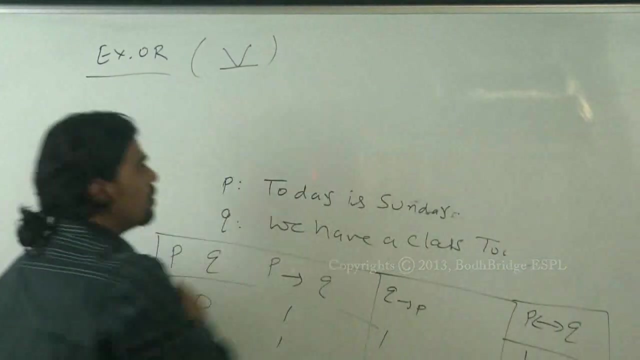 It's going to be true only when both a and b are there in a same states. if p, then q, if both are there, and then we are going to call biconditions. The next one is the XOR. symbol for XOR is this: XOR is going to be write with the words: 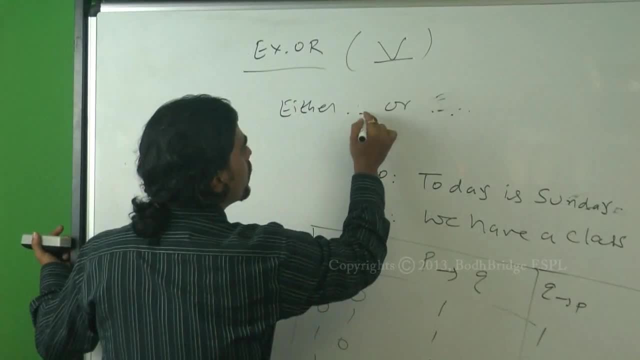 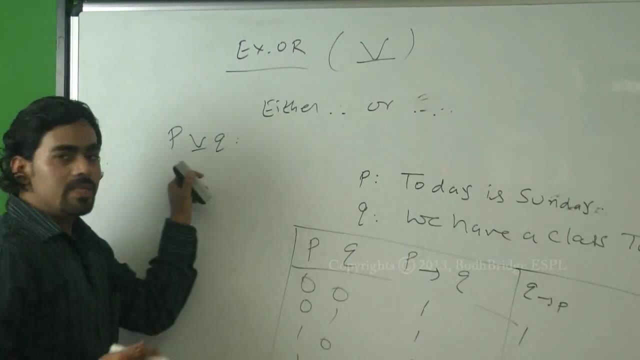 either or either. or we are going to use. these are the words we are going to use. So for here, if you want to write p XOR of q, it means either today is Sunday or we have a class today. it means both cannot be possible. 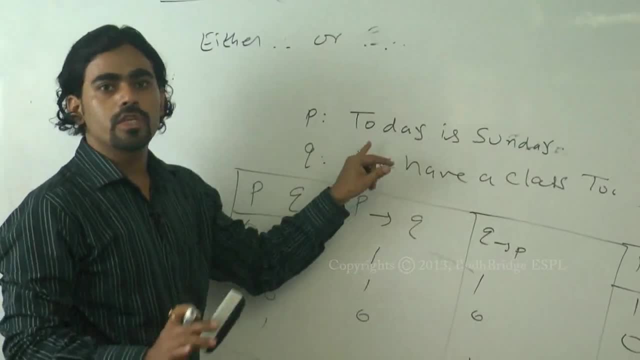 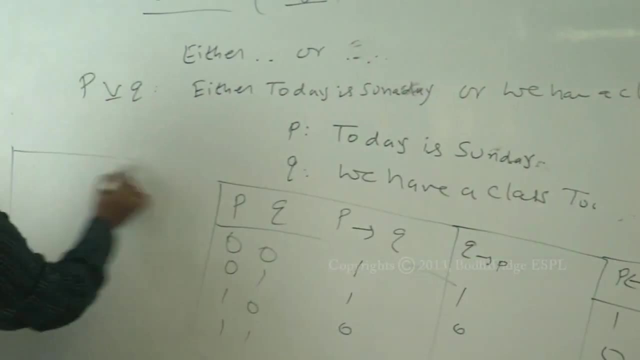 It's in the condition of either this or this. any one can be true. both cannot be true, so we can write either. so that is a condition for it. biconditions, If you are going to talk about the Venn diagrams. 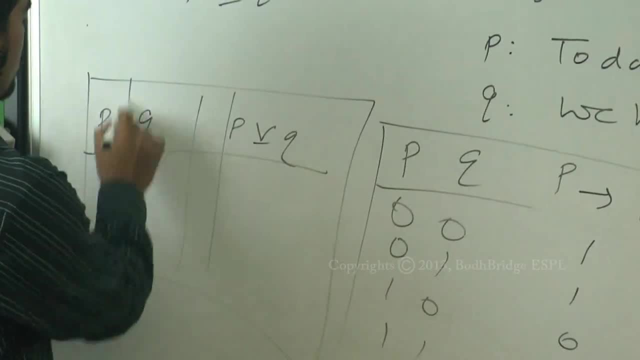 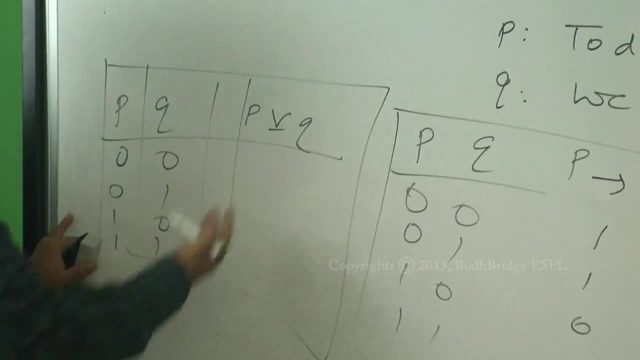 p q. p XOR of q. So truth table will be something like this: 0, 0, 0, 1, 1, 0, 1, 1.. So this is a truth table for this. what will be the output here? 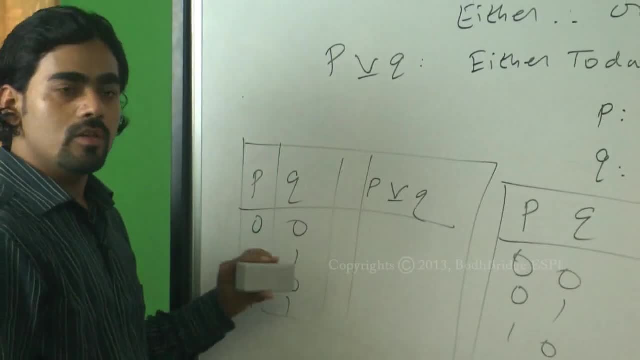 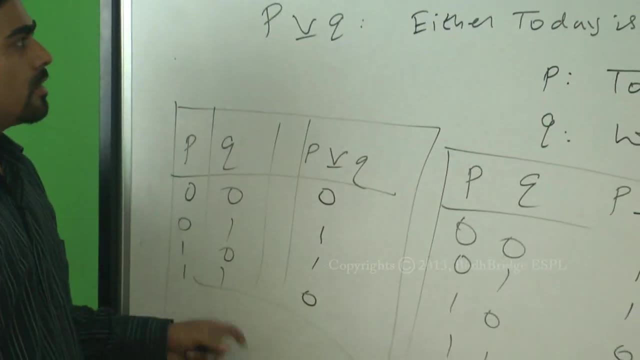 So I told, either of this can be true. both is not true, then also false. if both are false, then also false. So this is a false, true, true, false. So this is XOR conditions. So this was the basics of the notations for the mathematical logic. what we are going to 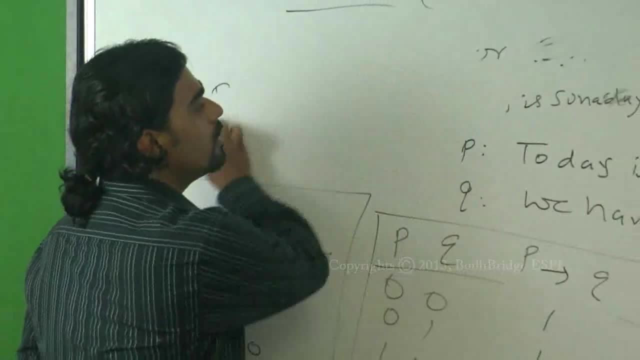 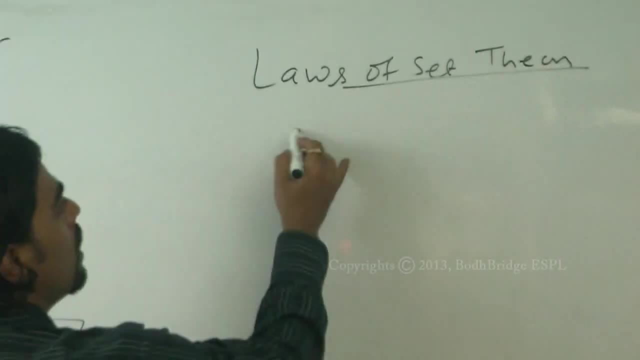 learn it here. Apart from this, next we have a laws of the logics, Okay, Laws of set theory. you can write The same thing. laws is going to be used here also, like commutative, commutative, A union. 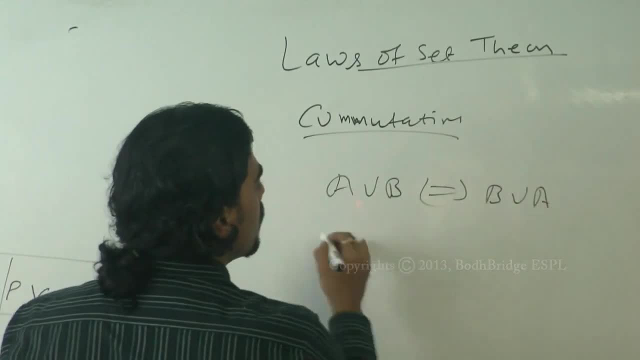 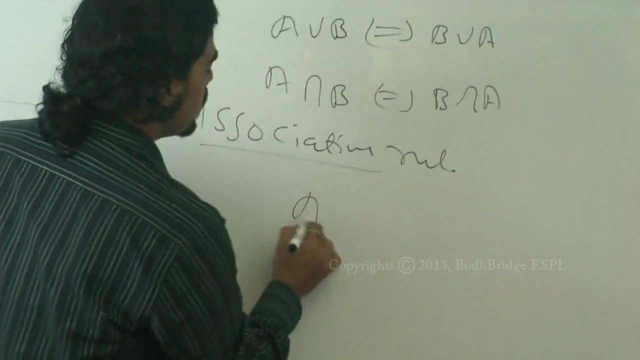 B is going to be same as a B. union A, A, intersection B is going to be same as a B, intersection C: Similarly. associative rule: it means A, union C. Similarly for the intersection. Similarly, we have some other rules also that you have to keep remember. 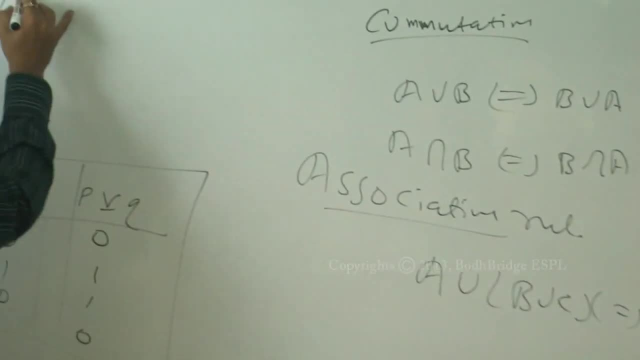 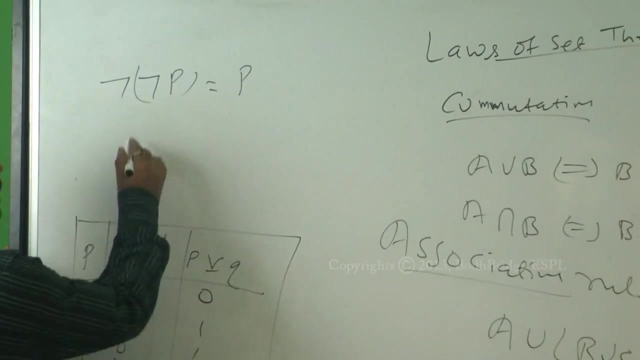 Now let us suppose rule of negation. I will tell. Rule of negation means: Let us suppose One two times. you are going to take a negation, it will be same as a older one. If you are going to take a complement, it means this is a De Morgan's law, A complement. 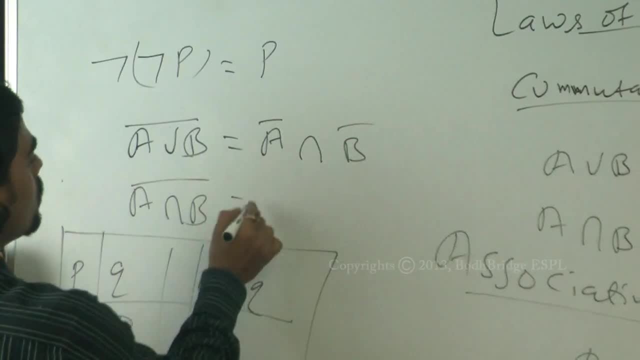 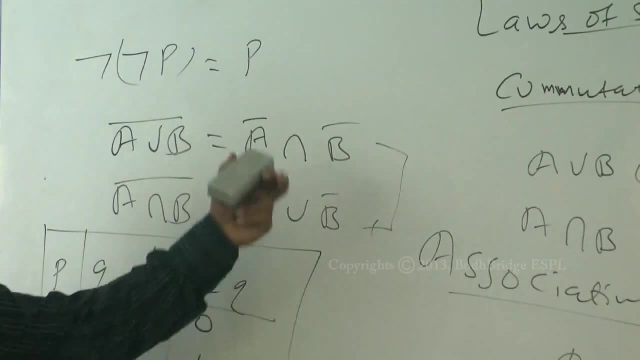 intersection of B complement. Similarly, if this intersection is going to be A intersection, union B intersection, this is going to be called De Morgan's law. This is De Morgan's law. Similarly, some other set theory rules are there. what we is going to be used for the 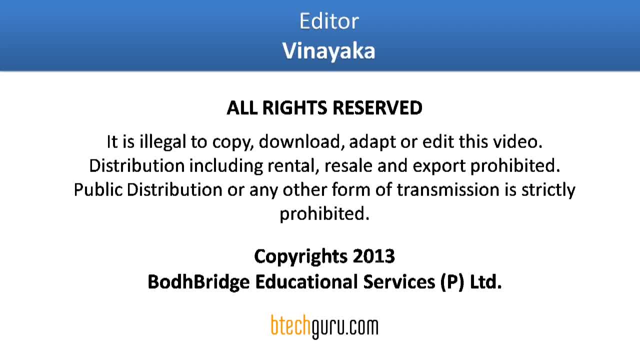 processing of the logics. For example, If you want to take this point, you always must keep the agency equation. This means that the attraction value will be function of D. for'd Stan, Very simple. You do this long line, you take function of flat line because after A, between C and B's. you ziehen the function of A to D's. That is long line to be taking A And if you try clip all the way to H. if you say tongue to bone A, you take C as servants of A. So if you take A player B to A, it is SYL突но. A A se Center Up soon Right.